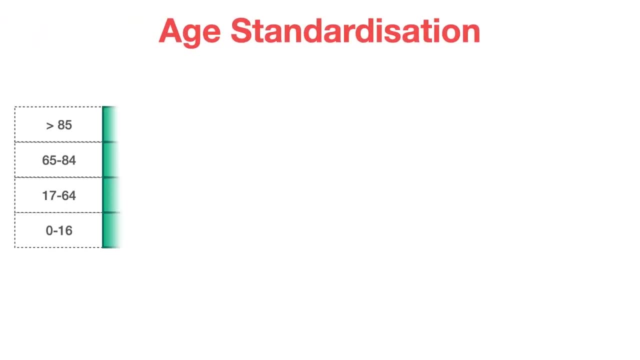 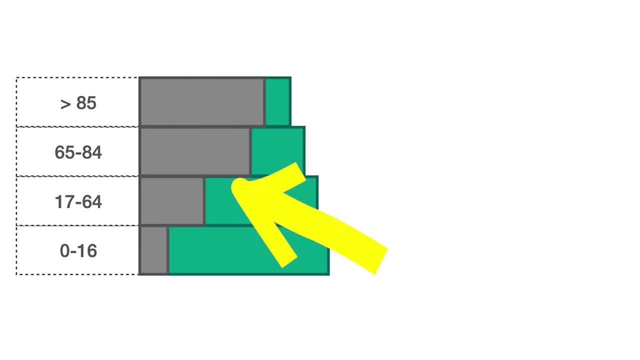 And let me illustrate the problem for you. Let's divide the population into age bands. The green bars represent the size of the population in Egypt. The green bars represent the size of the population in Egypt. The gray bars are the proportion of that group that die because of the disease that we're. 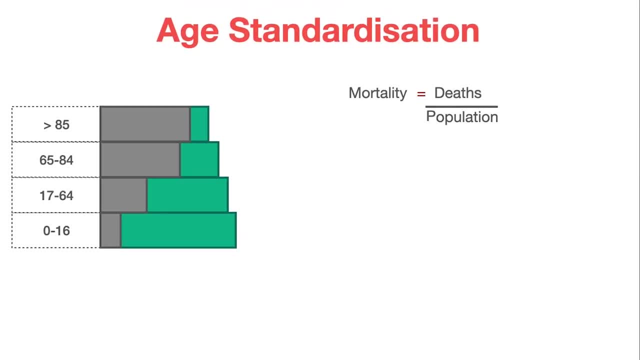 interested in Now. remember that we said that mortality rate is deaths per population, or the number of deaths divided by the population size. So it stands to reason, then, that the population size times the proportion of the people who die in that population the mortality will give you. 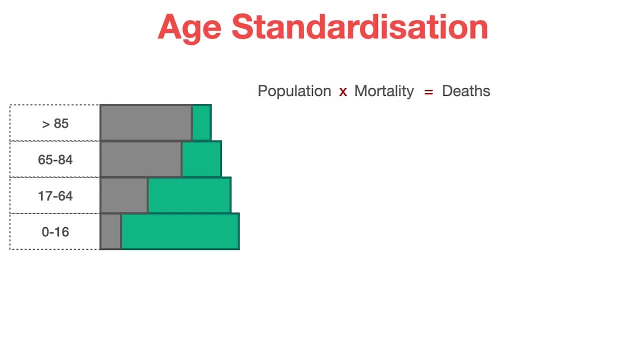 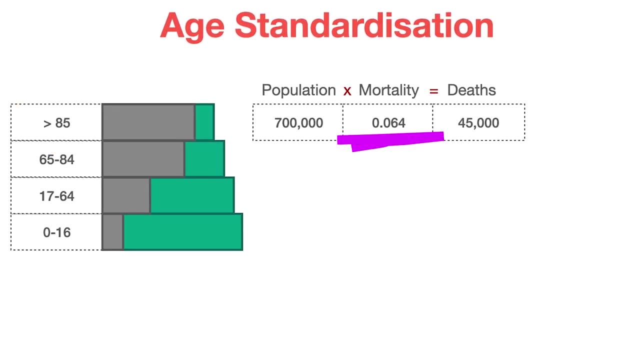 the number of deaths? right, Of course it's right. Easy peasy, lemon squeezy, Let's keep going. So 700,000 people over the age of 85, times the proportion of the population who die in that age group- 0.064,- gives you 45,000 deaths in that age group. And of course we can do that for all. 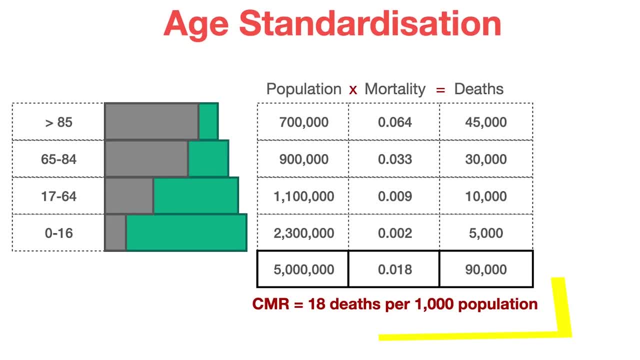 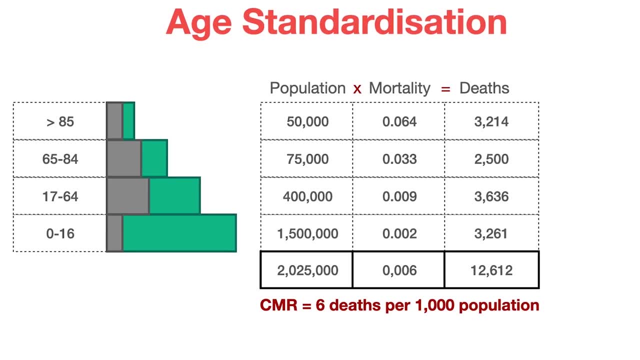 of the age bands. In this example we've got a crude mortality rate of 18 deaths per thousand population. Now let's see what happens if we change just the age structure of the population. Hang on, What's going on here? Now we've got a crude mortality rate of about a third of that. 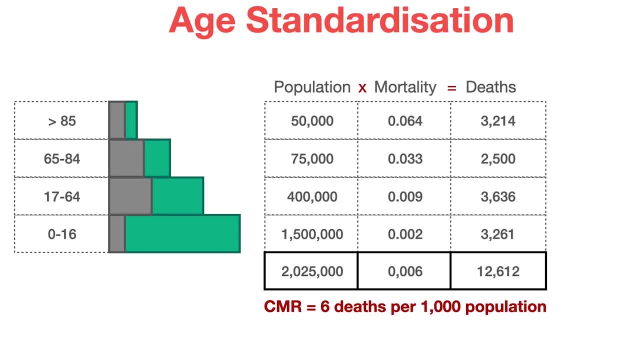 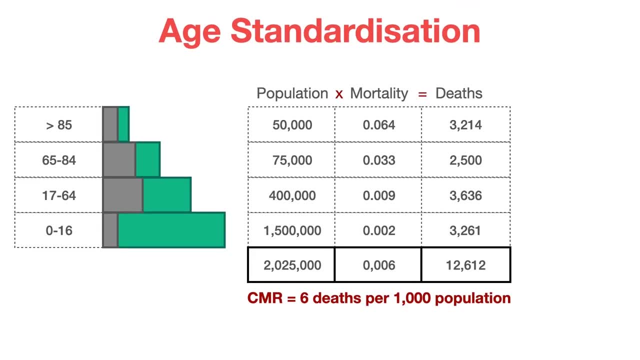 six deaths per thousand population, And all we've done is change the age structure. In these two examples, the mortality rate of the population is 0.064.. Now let's see what happens if we change. the rate of each age band has stayed exactly the same, And the lesson here is that age is a confounding 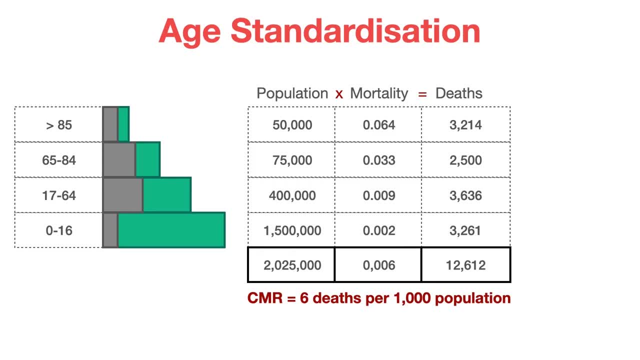 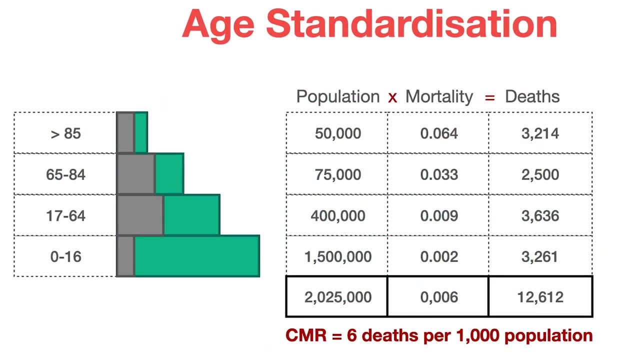 factor right. You cannot compare the crude mortality rate of two populations that have got different age structures. So what can we do to fix this? Well, I'm glad you asked. There are two strategies. There's what we call direct and what we call indirect age standardization. This is not. 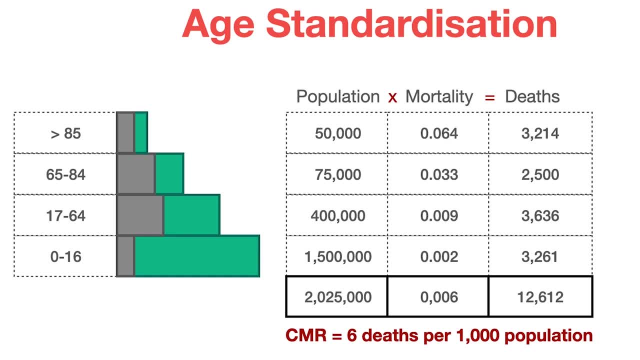 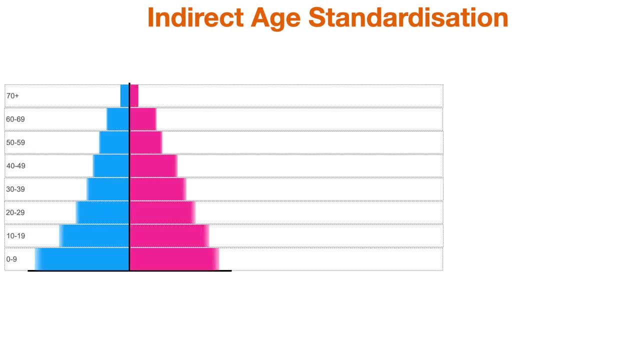 complicated. Stick with me, I promise you you're going to understand this Giddy up Right. We're going to start with indirect age. Let's imagine that we're looking at a country- Maybe it's a country like Ireland- And this is: 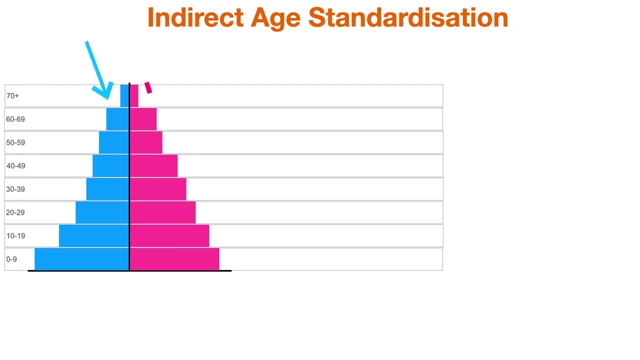 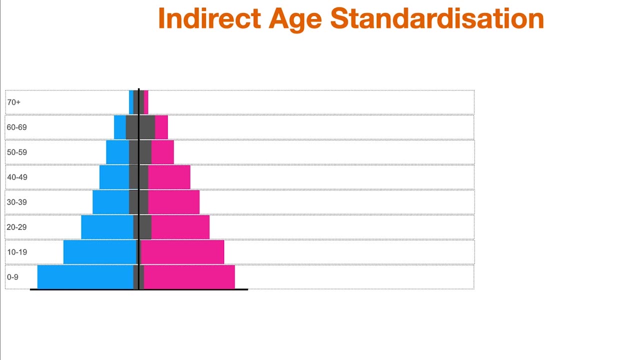 a population pyramid where men are represented in blue, Women are represented in pink, for each age strata. Now again, of course, the gray is the proportion of the people in each age strata that die. That's our mortality rate. And again, we've got a population size, We've got a mortality. 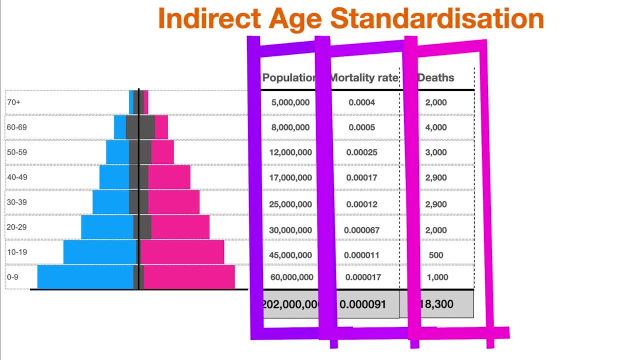 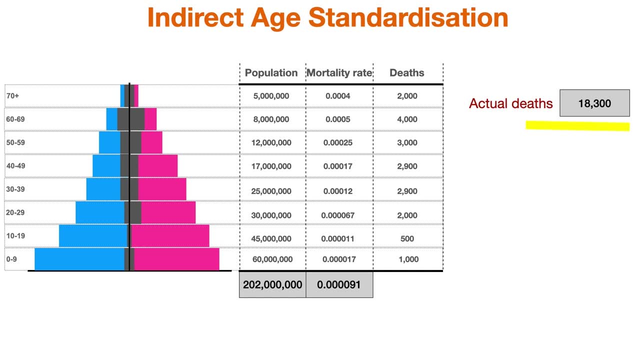 rate in Ireland And we've got a number of deaths right for each age strata. With me, Of course, you are with me, Let's keep going. We start off by noting the actual number of deaths in Ireland, and we want to know if that number is bigger or smaller than the number of deaths that you'd expect. 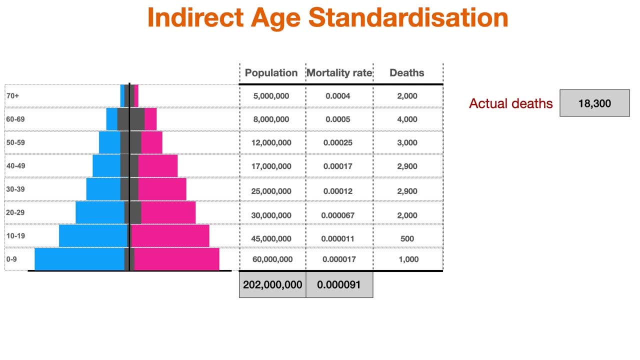 if Ireland had the same mortality rate as Europe as a whole. So let's remove the Irish mortality rates and the deaths and let's drop in a standard population mortality rate, in this case that for Europe, And then let's calculate the number of deaths that we'd see in each age strata and add. 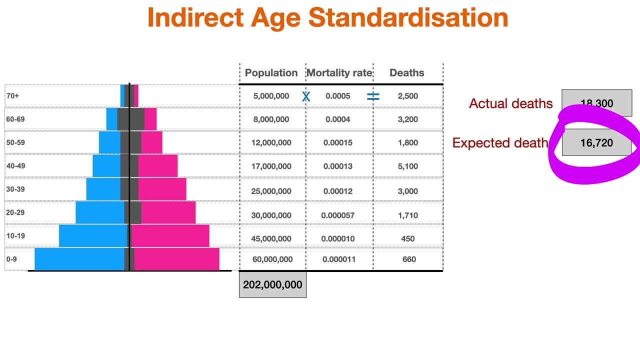 them up And this gives us the total number of deaths that we'd expect to see if it were the case that Ireland had the same mortality rate as the whole of Europe. And we can see just by looking at those two numbers that Ireland has more deaths than you would expect to see if it had the European 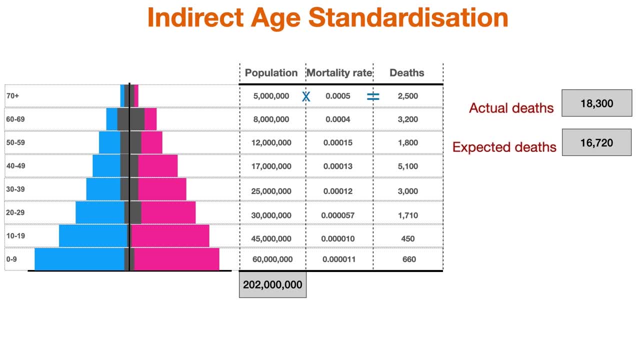 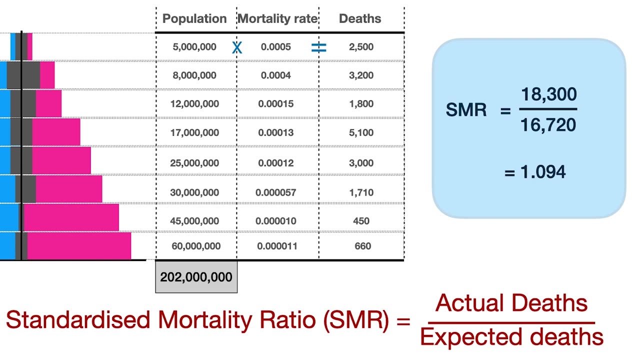 mortality rate applied to the Irish population age structure, And we can look at the ratio of the actual over-expected deaths, and this is called the Standardized Mortality Ratio, or SMR, And in this case the SMR is 1.094.. Now, if it was exactly one, that would mean that the actual 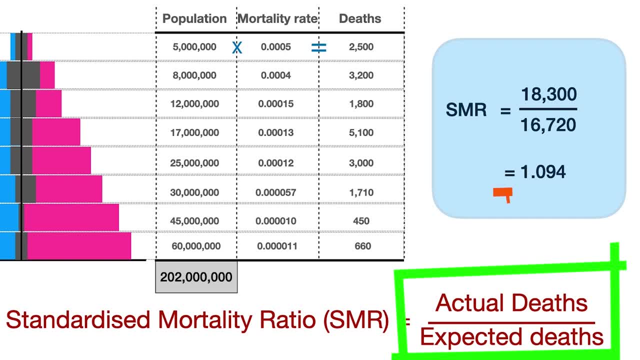 and the expected deaths were exactly the same. So we can look at the ratio of the actual and the expected deaths, and this is called the Standardized Mortality Ratio, or SMR, And in this case, exactly the same. The fact that it's more than one means that the age-adjusted mortality rate in 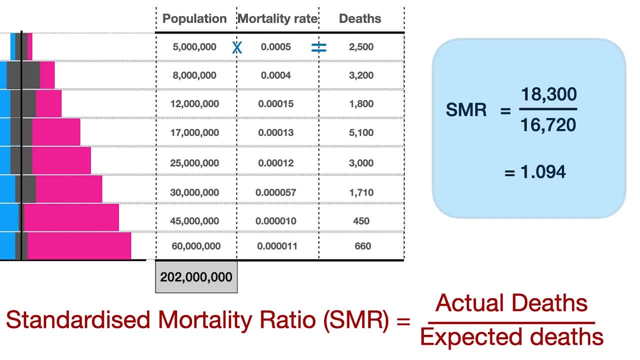 Ireland is higher than for Europe as a whole And of course, if it was less than one, then Ireland would have an age-adjusted mortality rate lower than for the whole of Europe. And of course we can apply the same technique to other European countries and compare their SMRs to see who is. 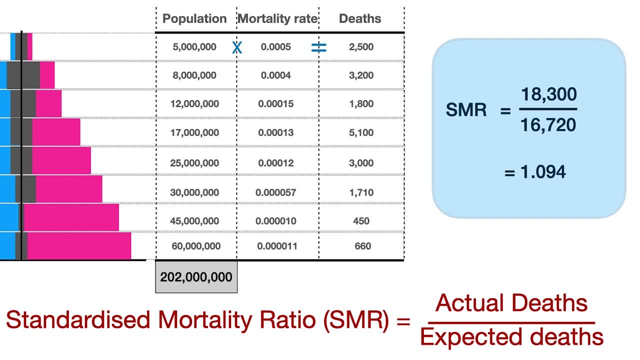 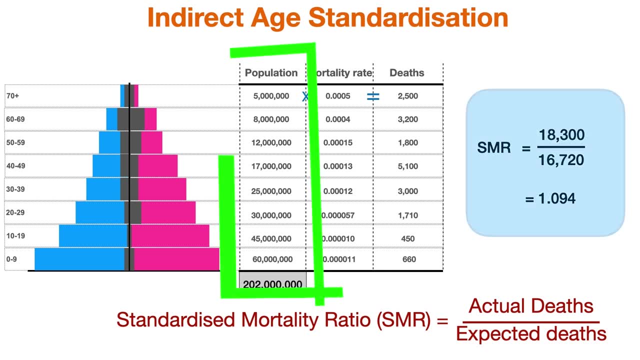 doing better. You got it, Of course you've got it. Let's keep going, Boom shakalaka. Okay, until now, we've been talking about indirect age standardization And to do that, take note of the fact that we left the population structure alone and we dropped in a standard. 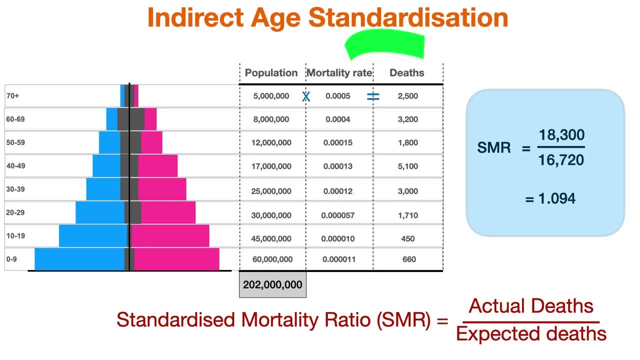 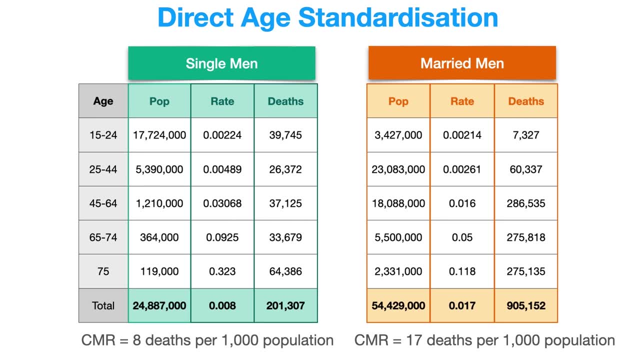 mortality rate and did the calculation and worked out sort of the expected deaths. Let's now look at direct age standardization. Here we're going to do something slightly differently, So just take careful note. Now we're going to compare the mortality rates of single and married men. 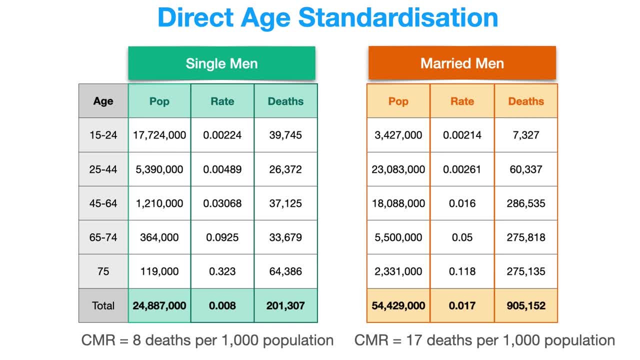 Super duper interesting. This time, instead of substituting in a standard mortality rate, we're going to keep the mortality rates of the two populations that we're comparing and we're going to drop in a standard population structure instead. Let's take a look at how to do. 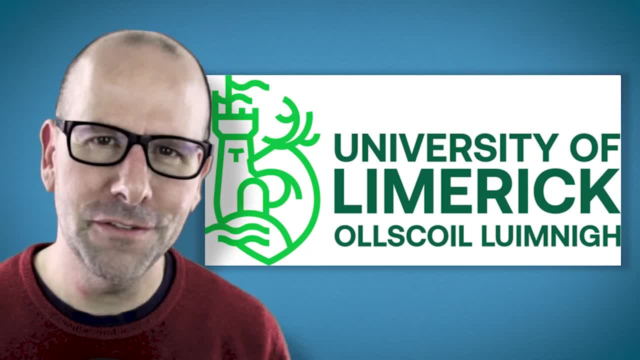 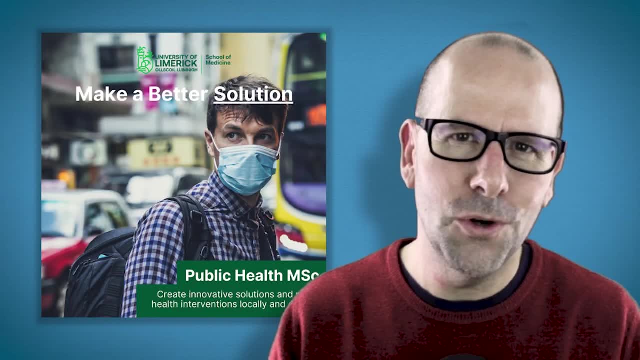 that, And before we carry on, a big thank you to the University of Limerick for supporting the creation of this video. The University of Limerick are offering an MSc program in public health which is absolutely world class. I actually think it's one of the best master's level. 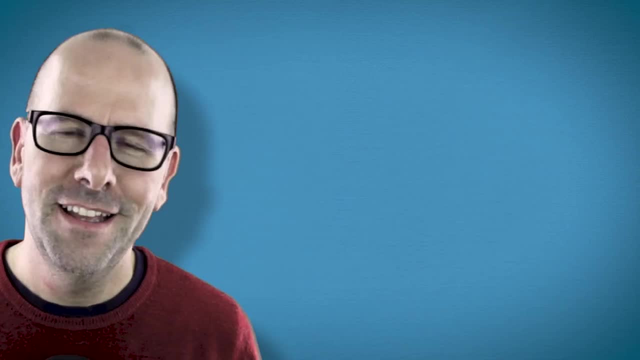 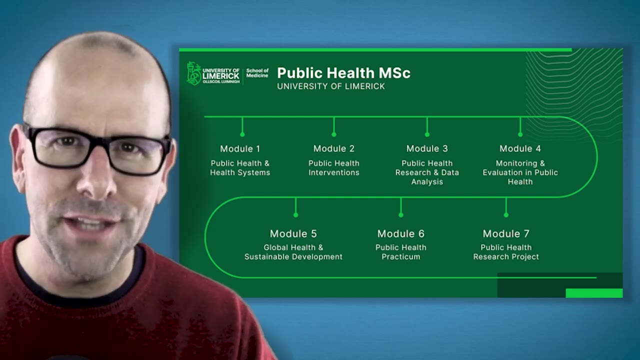 public health degrees that you can get anywhere on planet Earth. The program they've put together has been very specifically and carefully designed to prepare the graduates for work in the global health space. Now it's a new program, but it's very quickly getting a reputation for. 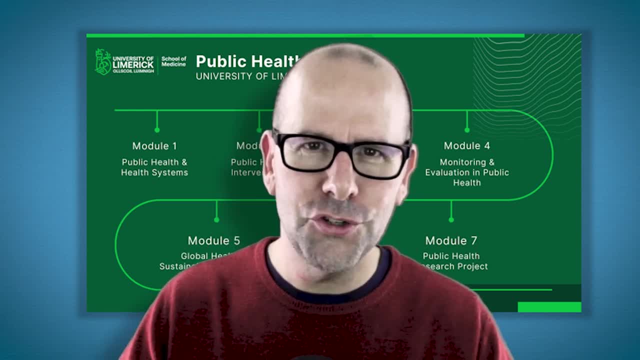 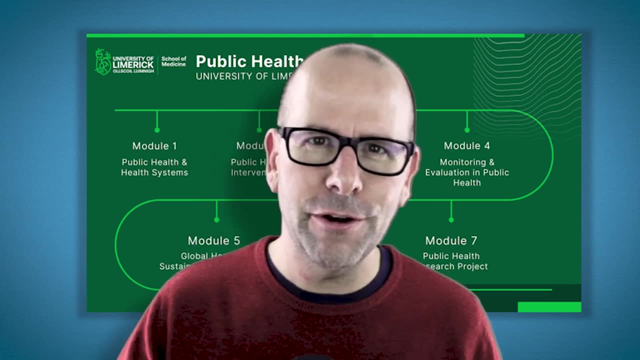 being one of the best places that you can study public health if you want to be properly prepared for a job in the workplace, And it's certainly going to get a reputation, before you know it, as the place that people that are employing public health graduates look to for very strong workforce. 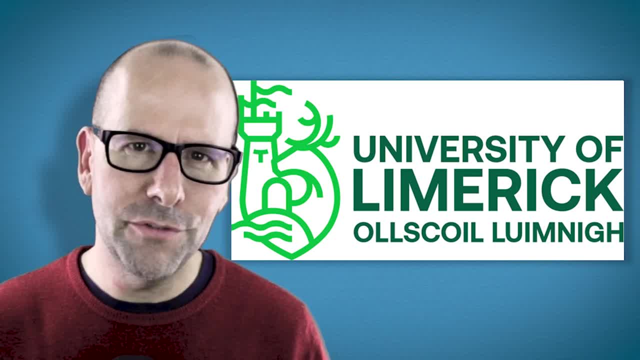 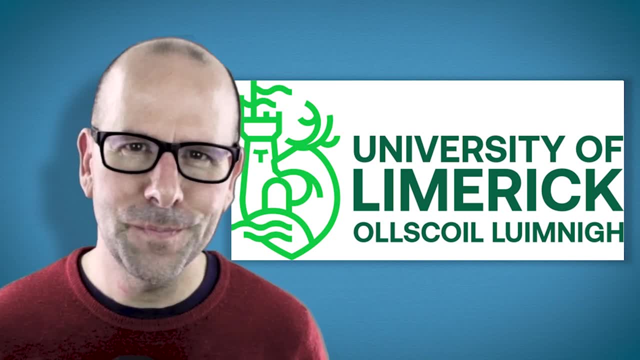 candidates. You can do it full time over one year or do it as a part time program over two years. Highly recommended, Definitely check it out. I'm going to put a link in the description below. Okay, let's get on with this video. In these two groups, the crude mortality rate. 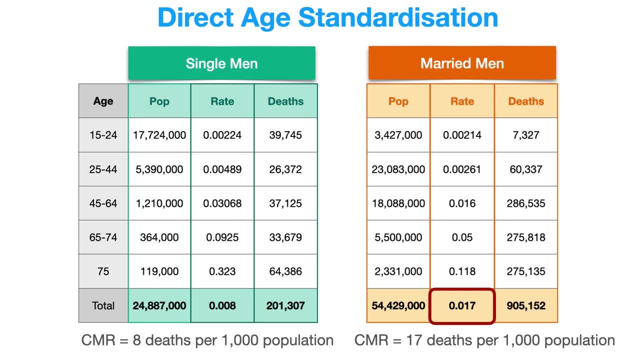 in married men is 0.017 or 17 deaths per thousand population, which seems to be about double the crude mortality rate of single men, which is at eight deaths per thousand population. So, before adjusting for age, it looks as if single men are much healthier than married men. Huh, Let's take 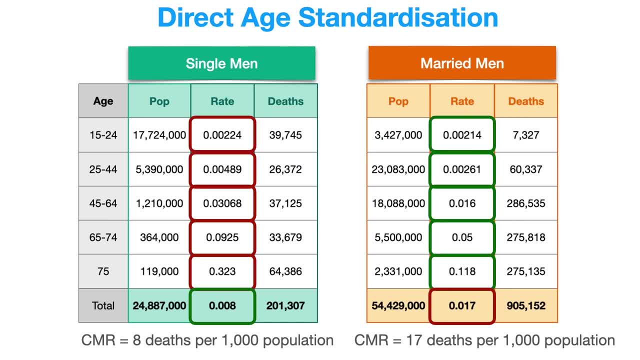 a look if that's actually true, once we've adjusted for age. In every single age band, single men have a higher mortality rate than married men And the reason for this is because they have a higher mortality rate than married men And they have a higher. 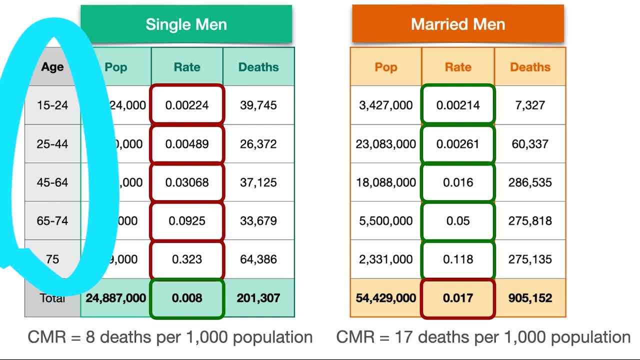 mortality rate than single men. The overall lower crude mortality rate is, of course, that the age structure of single men is very different than for married men, right, There's a lot of single men who are young, where the mortality rate is low, And there's a lot of married men who are older, where 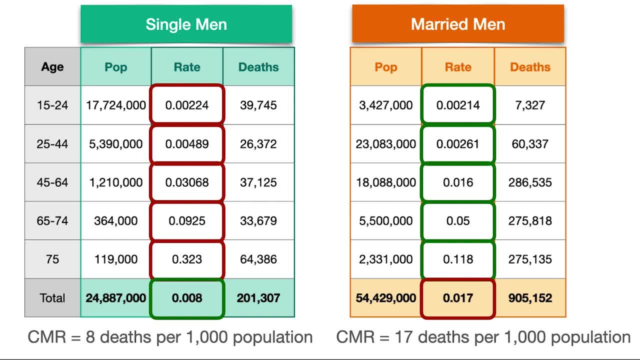 the mortality rate is higher. So, for example, in the over 75s, despite the fact that single men have a mortality rate three times higher than married men, because so many of the over 75s are married, the actual number of deaths amongst married men in that group is much higher. And 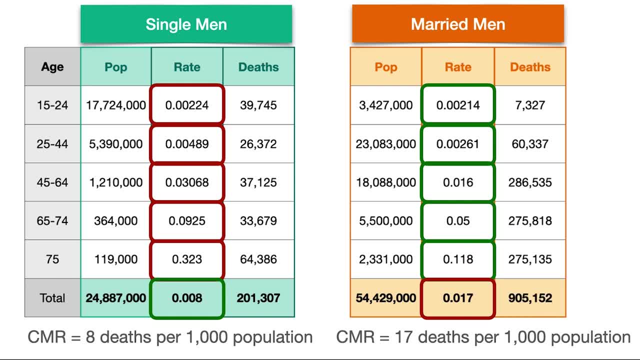 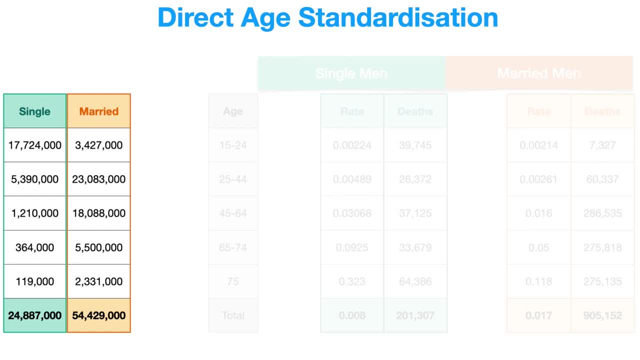 again, the age structure is a confounding factor, So let's look at how to control for it In direct age standardization. we're going to say: look, let's imagine that both groups have got exactly the same age structure right, So we're going to take out the age structure that we've 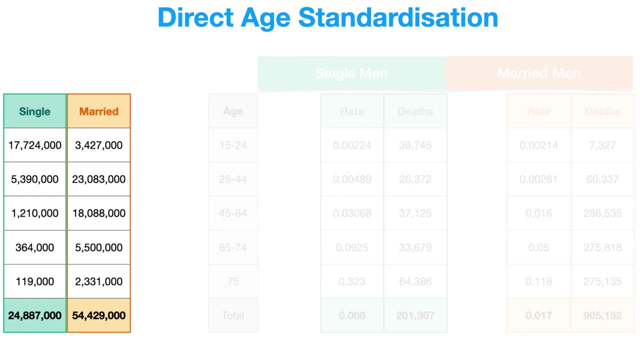 got and we're going to pop in a standard age structure And by doing that we're controlling for age. Age structure can't possibly influence the comparison, because both groups are going to have the same age structure. right, We could use any standard age structure for this. 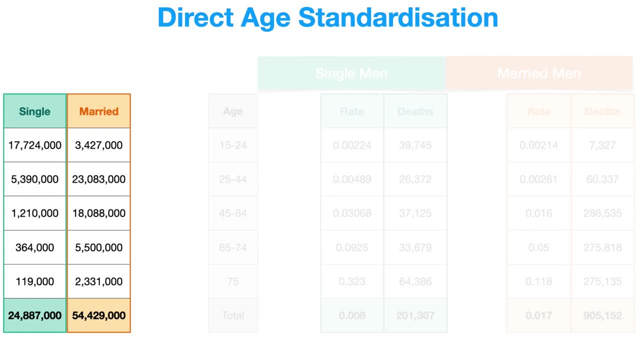 and drop it into the two tables. That would be fine, But in this case, what we're going to simply do is we're going to add up the two groups that we've got. add them together, because if you've got single men and married men, all together, 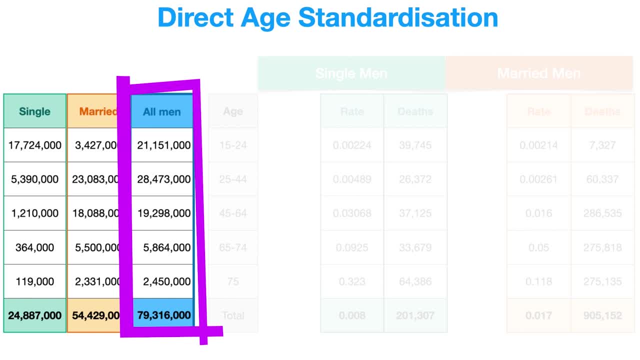 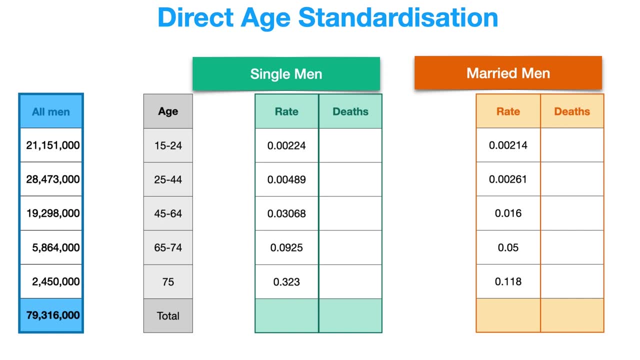 they make up all men in the population and that becomes our standard population and we're going to use that age structure. Now we're going to take that standard population structure and we're going to drop it into both tables, right for single men and married men. 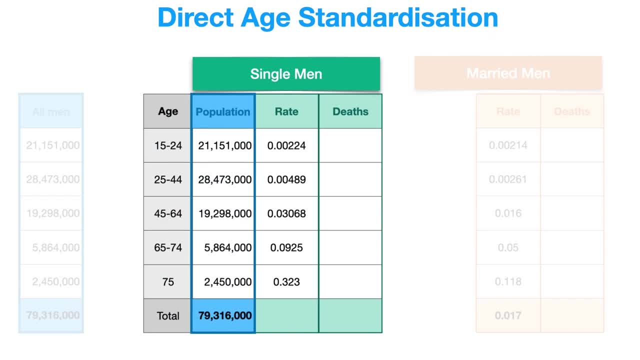 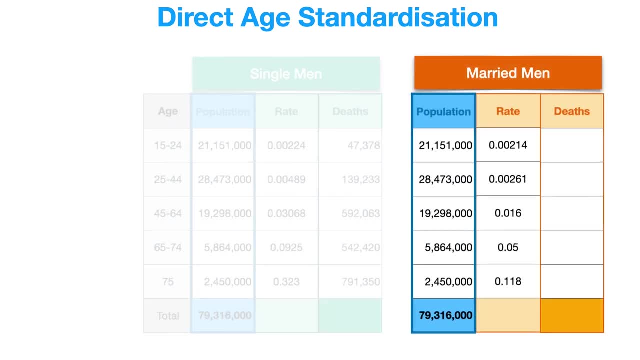 and calculate the number of deaths that we would expect, right, So we drop it into the single men table and we calculate the number of deaths that you'd expect. and we drop it, in the standard age, in the standard population, into the married men table and, of course, we calculate the number of. 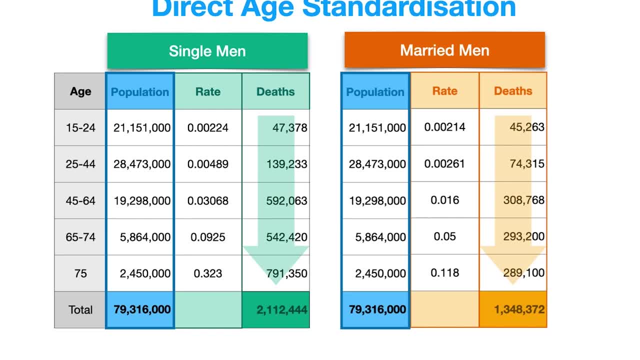 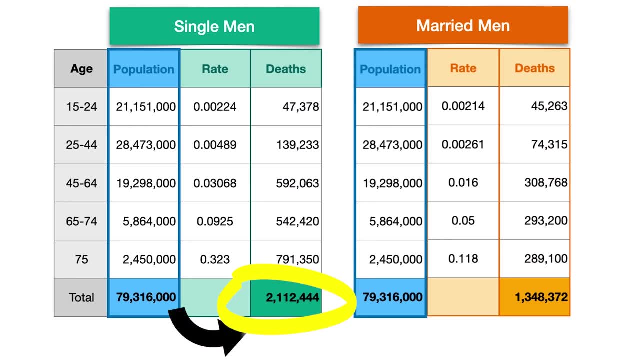 deaths that we'd expect in that group, and then we add them up and we get a total number of expected deaths in both groups right Now. remember that mortality rate is deaths divided by population, and so, of course, now we've got ourselves, voila, an age-adjusted mortality rate in each group that. 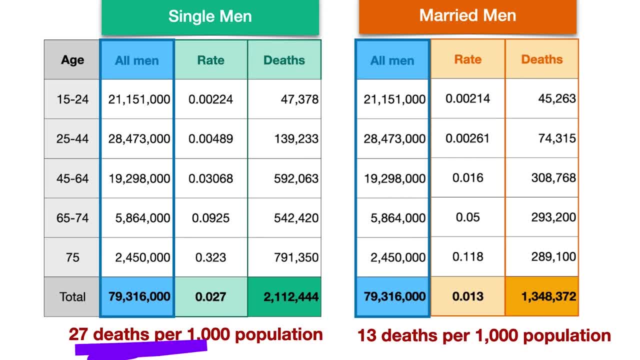 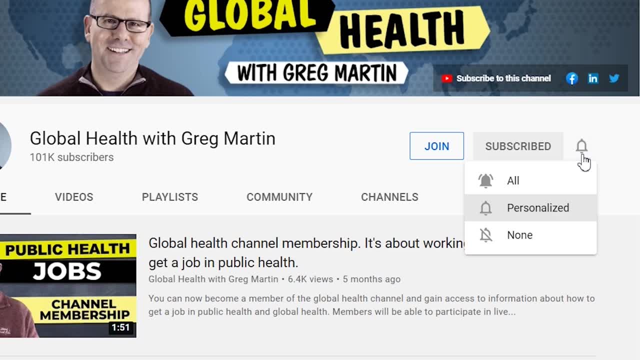 can be compared. Isn't that amazing? So single men have an age-adjusted mortality rate of more than double that of married men. Stay and watch another video. Subscribe to this channel if you haven't already Hit the bell notification to get notifications of future videos in the future. 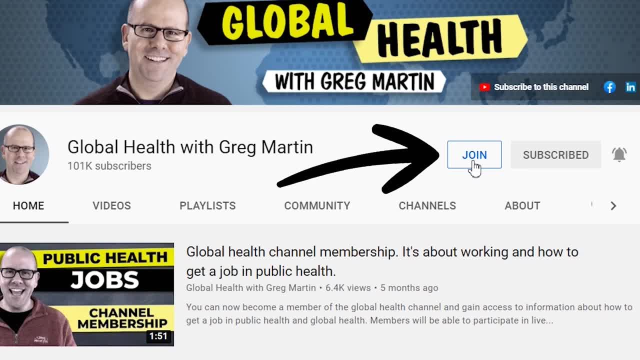 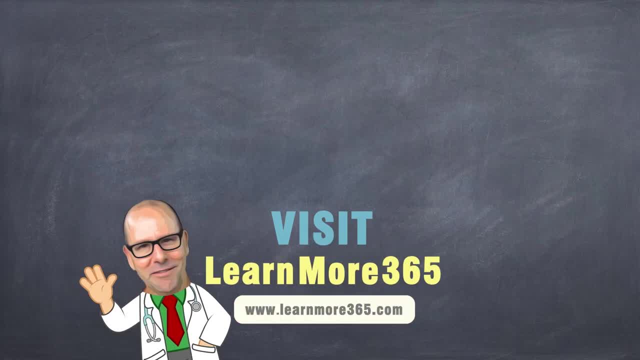 Consider becoming a member of the channel. I create members-only videos about jobs in the global health space, in the public health space, and for more teaching videos, go to learnmore365.com. Thanks for watching this video. I hope you enjoyed it. I hope that was useful. Don't do drugs Always. 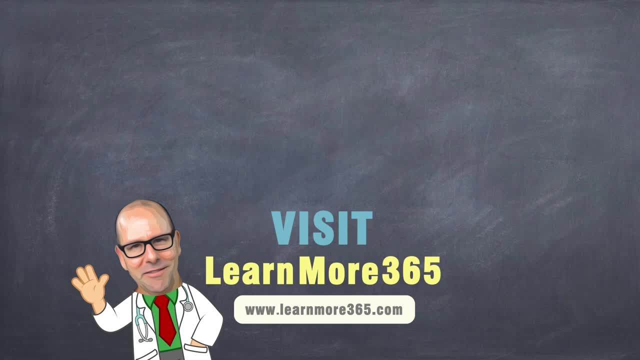 do your best, Don't have a change. Speak to you soon. See you here again in the near future. Bye.